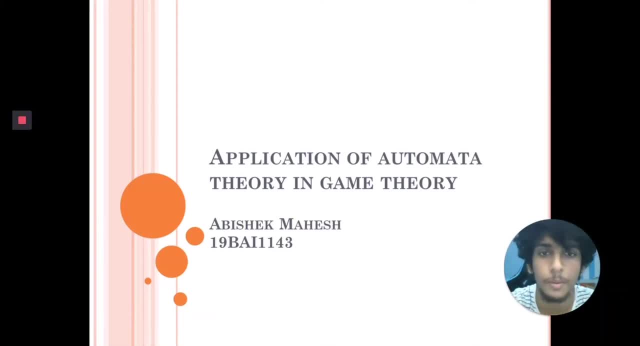 I'm Abhishek and I chose the topic of application of automata theory in game theory, and so we are going to see how automata theory is applied in game theory using various types of automata, such as finite set automata, adaptive automata and cellular automata. So we'll move on forward and 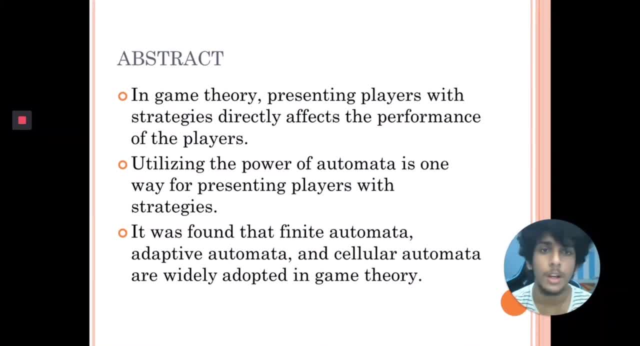 the abstract of this project is in game theory, presenting players its strategies directly affects the performance of the players and utilizing the powers of automata is one way for presenting players the strategies. So later it was found that finite automata, adaptive automata and cellular automata are widely adopted in the game theory and I have attached how these 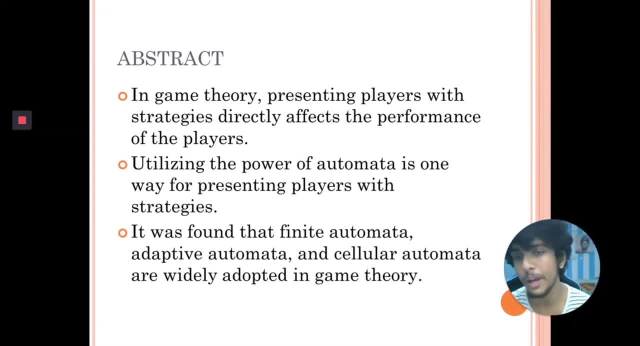 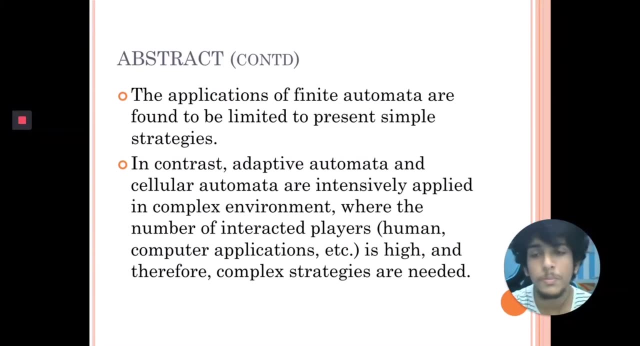 automata are applied in the game theory at the back of the slide. So I have given a detailed explanation on how finite, adaptive and cellular automata are used in game. So the applications of finite automata are found to be limited to simple strategies. So, in contrast, adaptive automata- 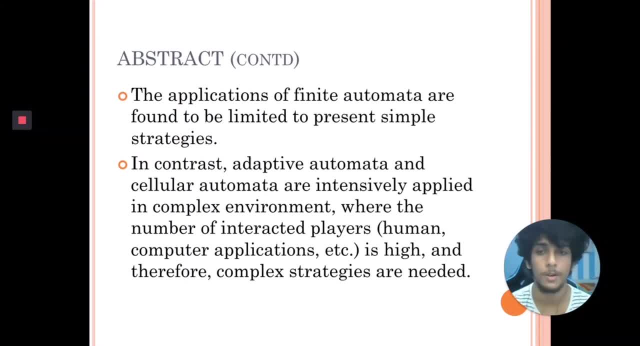 and cellular automata are intensively applied in a complex environment where a number of interactive players, like human and computer applications, is high and therefore complex strategies are needed. So basically what the thing is? finite automata are found to limited to be presented in a simple strategy. 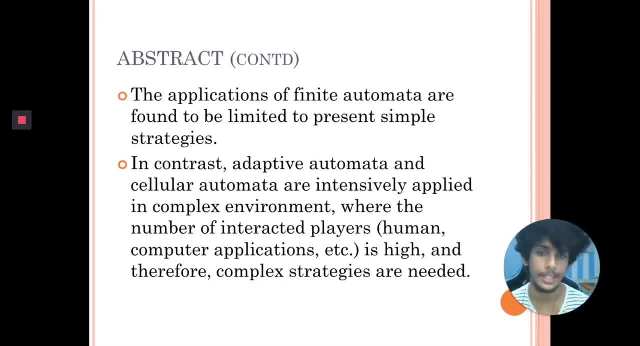 Whereas adaptive automata. adaptive and cellular automata are intensively applied in a complex environment. so, while building a complex game, we tend to use adaptive automata and cellular automata, whereas while developing a basic game in a well, while we develop a basic game- we are adapting the use of finite. 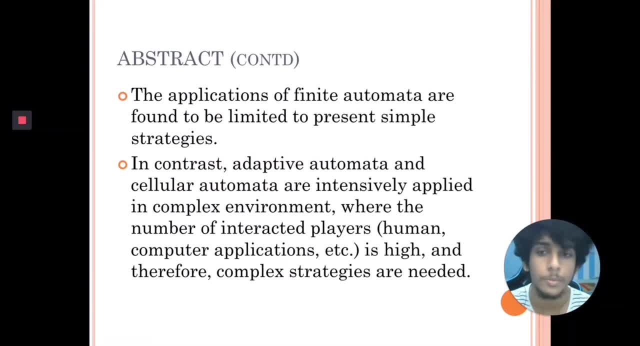 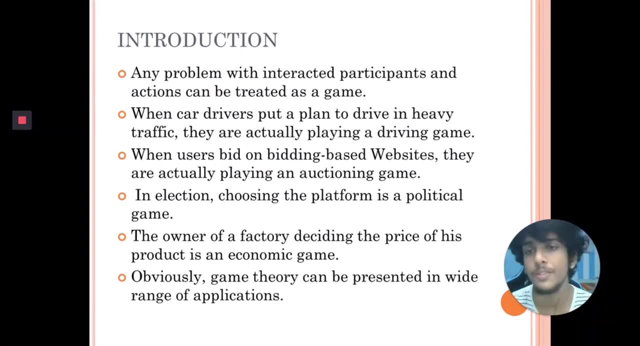 automata in it. so i have attached the use of finite automata and adaptive automata as regarding to my research in the back of the slide. so yes, so we'll start off with the introduction. so the basic introduction of the project application of automata and game theory is. so any problem with. 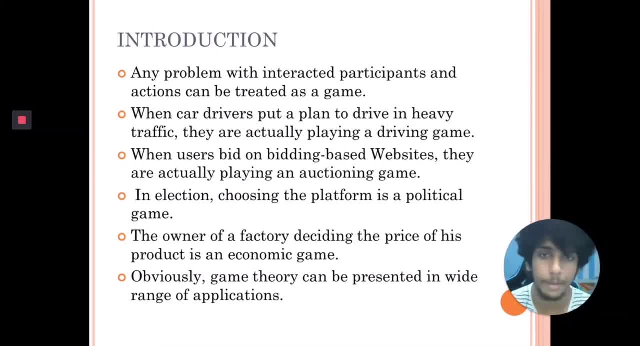 interacted participants and actions can be treated as a game. so anything, anything can be treated as a game. so when a car driver puts a plan to drive in heavy traffic, they are actually planning to driving a game. they are actually playing a driving game. so when users bid on a bidding based 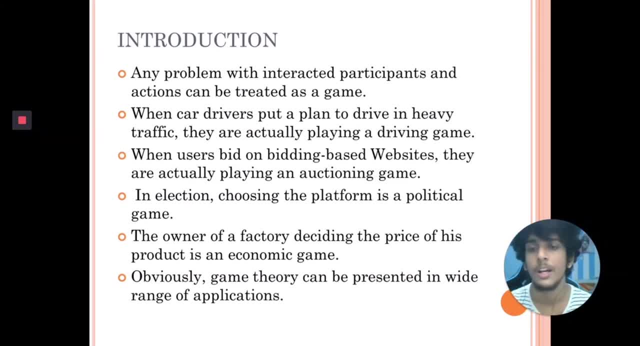 websites. they are actually playing an auctioning game in election. choosing the platform is a political game and the owner of the factory deciding the price of the product is an economic game. obviously, game theory can be present in a wide range of applications. i have limited my example to some five points where this gives an basic idea on what a game theory is and how. 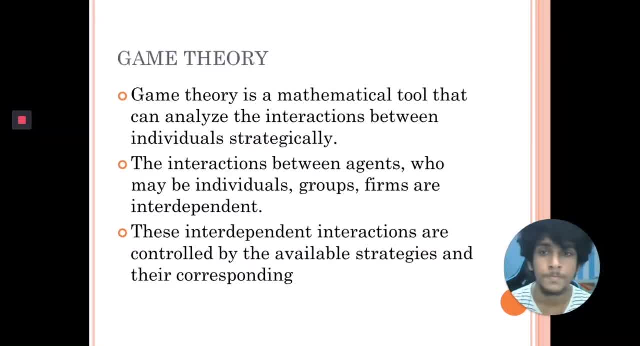 automata is applied in a game theory. so yeah, i'll give you a brief definition on what is game theory. so game theory is a mathematical tool that can analyze the interactions between the individual strategically, the interactions between agents, who may be individual groups. firms are independent. these interdependent interactions are controlled by the available strategies and their corresponding 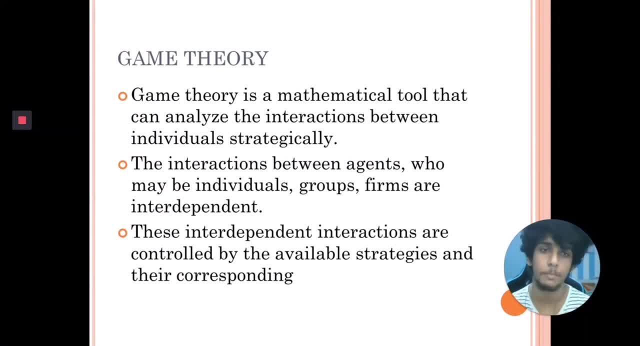 strategies. so basically, game theory is a mathematical tool which can analyze the interactions between the individuals. so if there are certain individuals who are trying to play a game on team mode, this game theory interlinks the different people's in a game. so this is basically the principle of the game theory. so game theory it's just a mathematical algorithm or tool. so the 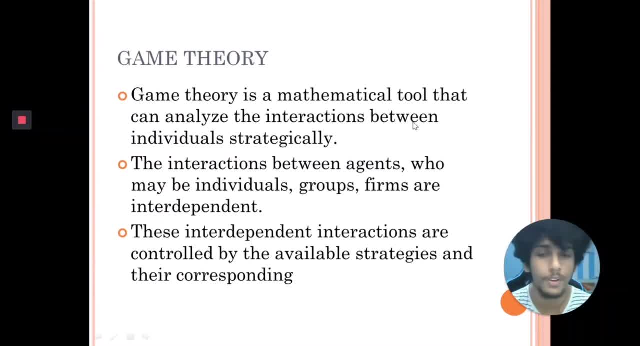 interactions between agents, who may be individuals, groups of firms, are interdependent, and these interdependent interactions are controlled by the availing, i mean the control by the available strategies. so if you take it that, uh, the strategy is a game theory and the game theory is a mathematical. 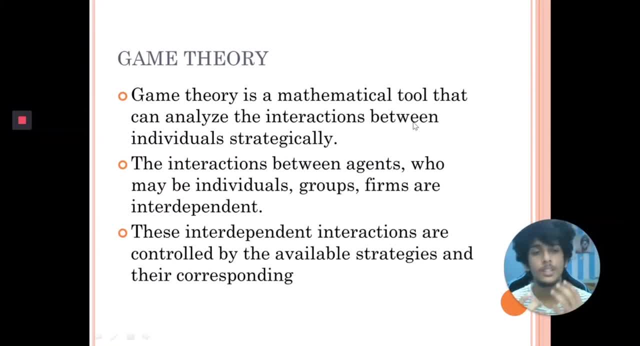 tool that can analyze the interactions between agents, who may be individual groups. firms are interdependent, and while now i think game theory is really important while playing a game. so if you apply the correct and the exact strategy, you can- i mean you can- get success on the game. so 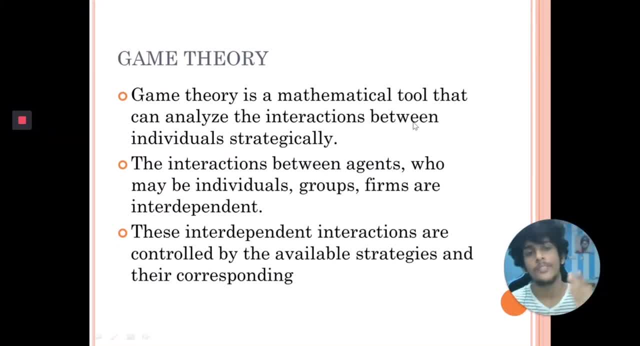 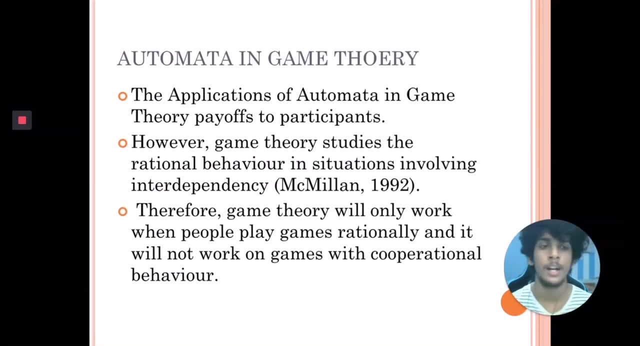 more like cracking an algorithm, or i mean game theory is nothing but an algorithm, or the players who are playing will crack the algorithm and will reach to the final position. so these are the inter. yeah, now i'll tell you about how automata is used in game theory. so the application of automata and 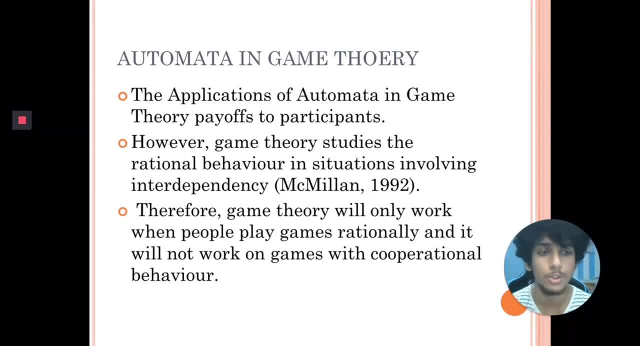 game theory pay off to the participants, so the participants are the one who are going to apply automata in the game theory. however, game theory studies the relational behavior in situations involving the interdependency. i came across this quote- game theory studies the relational behavior in situations involving the interdependency, from the book called macmillan in the year 1992. 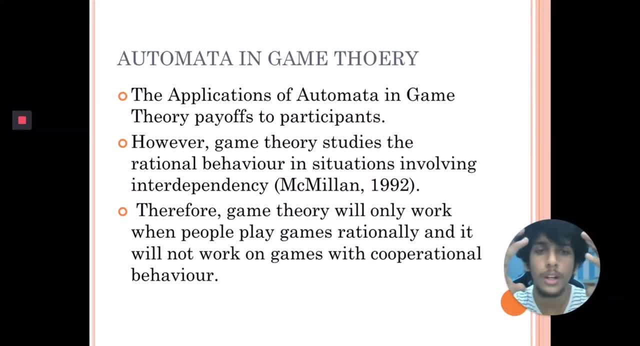 so this quote i mean uh, defines the whole thing on what automata is used in game theory. so game theory studies the relational behavior in situations involving the interdependency. that is the basic idea of game theory, which is using the automata. so therefore game theory will only 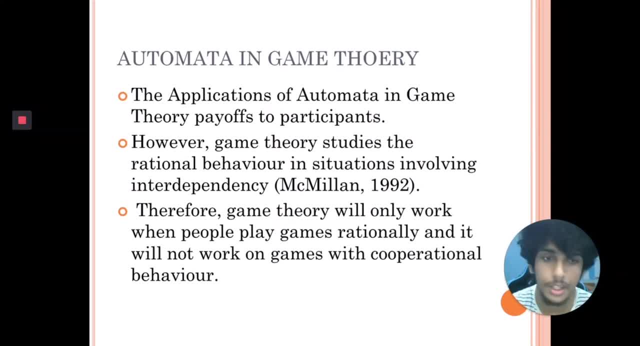 work when people are using the automata in situations involving the interdependency, when people play games rationally and will not work on games with co-operational behavior. uh, a co-operational behavior is nothing but where people form teams inside the game, where different people come across as a unit and they'll form a team and they'll reach the success point. but 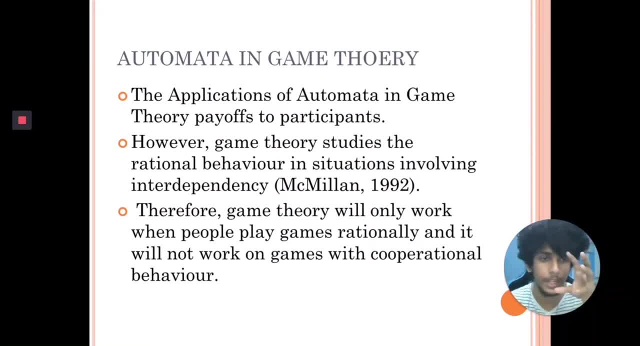 game theory will not work when people play games rationally. rationally means like uh, if they split up into different ratios and proportions, the game theory won't work. it will, uh, not work on the games with co-operational behavior too. so we'll check on where it will work, and generally, the game theory consists of the following entities: 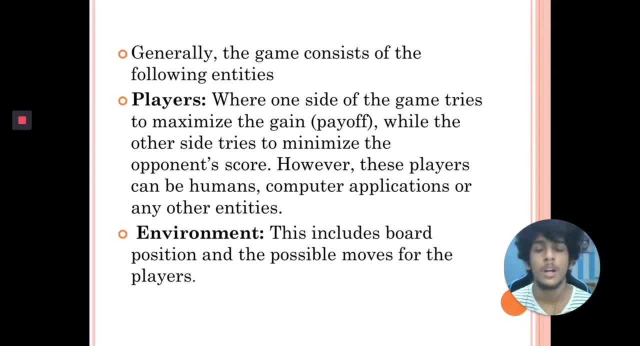 so, uh, there will be these following entities. so entities are the people and the environment and the things who are going to adopt the game. so there are these many kinds of entity in the game. they are players one, environment, two, successor function three, terminal test four. so now we'll check on the 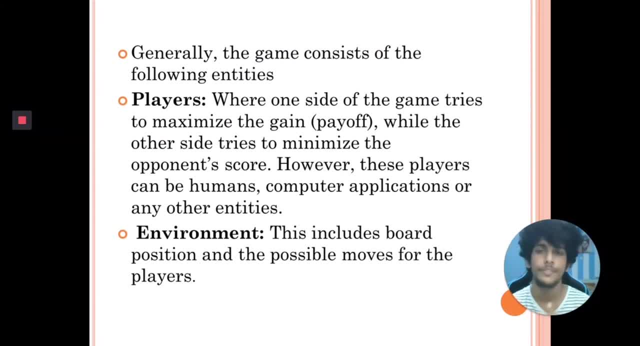 we'll check on the details of different entities where we are gonna study. so first entity is the players, the basic. as i have said above in the previous example, players are the one who are going to adopt art automata in the game theory. so where? okay. so what is the player? entity is: 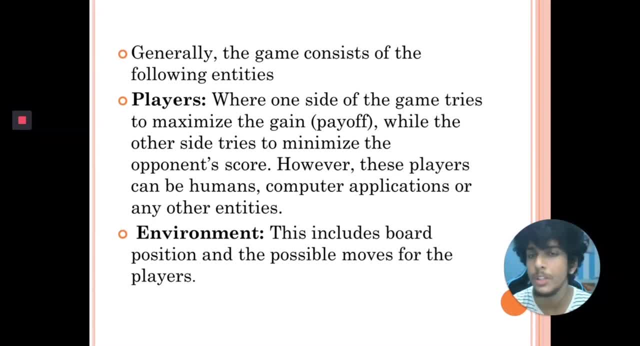 where one side of the game tries to maximize the gain payoff, while the other side tries to minimize the opponent's score. however, these players can be human. they can be robots, computer applications and any other entities, so players are the one who are trying to maximize the gain. 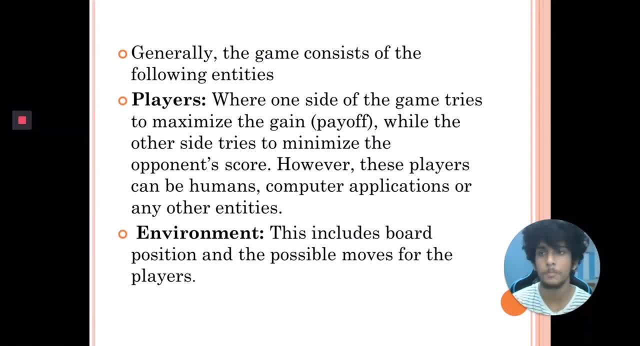 gain is nothing but the payoff or the points. you can say more as a point- while the other side- so there will be a collision between two sides- and the one who cracks the automata and cracks the algorithm reaches the final. so this is nothing, but, however, these players can be human, these humans. 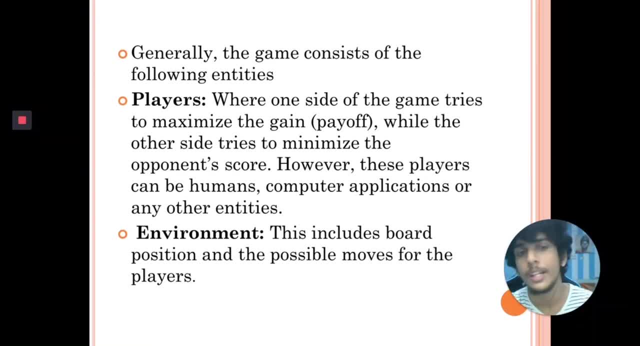 robots and completely computer applications can try to maximize the gain. so the whoever tries to maximize the game will reach the succeeding point. so the other entity is environment. so this environment, i mean this- is a. i mean this includes board position and the possible moves for the players. so 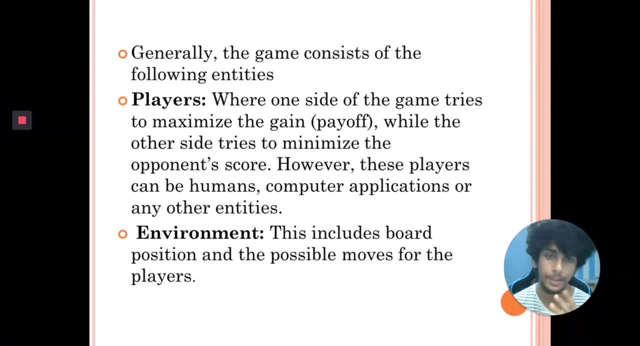 environment is nothing but the ui, the user interface, which includes board position and the possible moves for the player. so, uh, i mean, if you are playing a computer game or a basic game, uh, you'll dependent, you'll be, you'll be dependent on arrows. so the arrow key plays a major role in 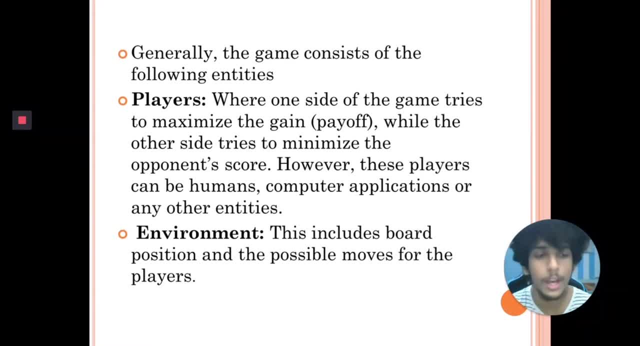 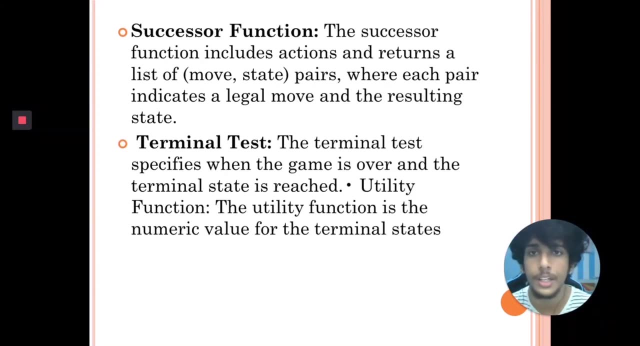 environment. so there'll be up arrow, down arrow, and side arrow, left arrow, left hand side arrow, right hand side arrow. so these arrows- i mean the thing which supports the players- are called as environment and the successor function is a other entity. so the successor function includes the actions and returns a list of moves, which is a state or a meaning, which is a move or a. 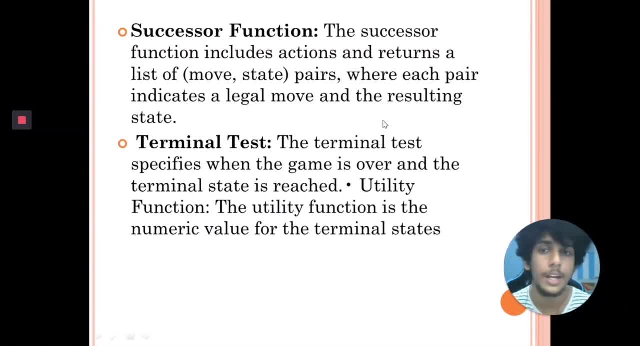 state in pairs, where each pair indicates a legal move on the resulting state. so, uh, i mean, this is a function which returns a list of moves, suppose in a suppose if you are playing a running game and if you want to move forward and you want to come backward, so 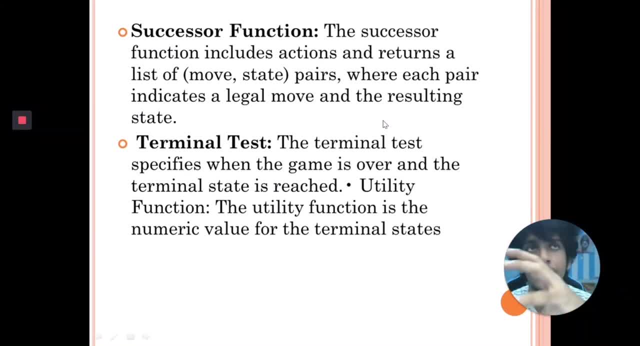 successor function will return the. i mean it will return the value. i mean, if you are moving forward, it will return you the forward thing, and if you are moving backward, it will return you the backward thing. so this forward, backward are paths where each pair indicates a legal move on the resulting. 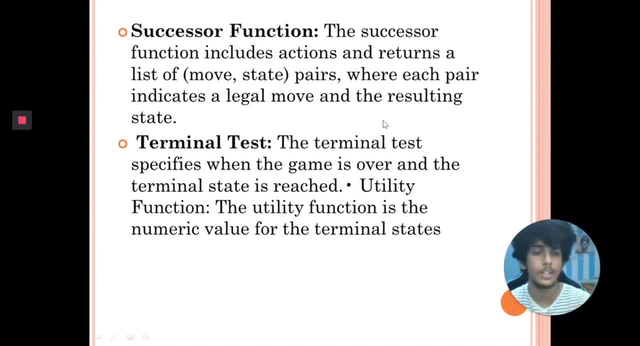 state. so if you move forward, the resulting state is forward, if you move backward, the resulting state is backward. so thus, that is the basic idea of a successor function. so then comes the terminal test. the terminal test specifies when the game is over and the terminal state is reached. utility: 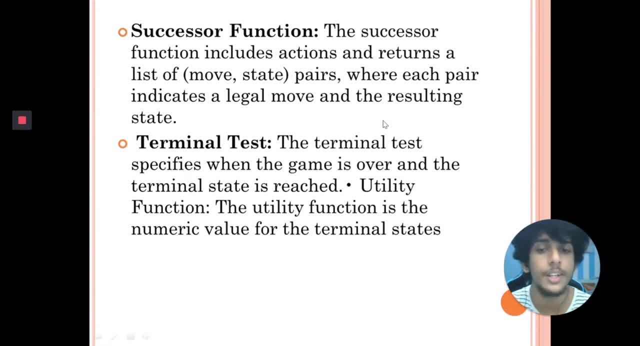 function, utility function. this utility function is the numeric value for the terminal states. so this terminal states and utility function are more or like correlated. so how we can say, like it is the union of terminal state or you can say the intersection of the terminal state. so the 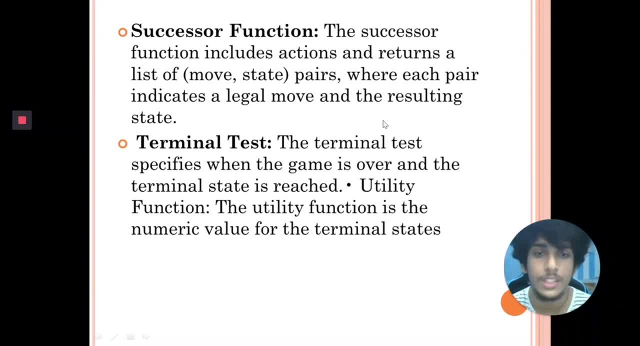 terminal test specifies: when the terminal state is EuroUSD, code is realized. so this is the. the game is over and the terminal state is reached. so the utility function is the numeric value of the terminal state. so in the automata theory of the game there will be two values called as zero. 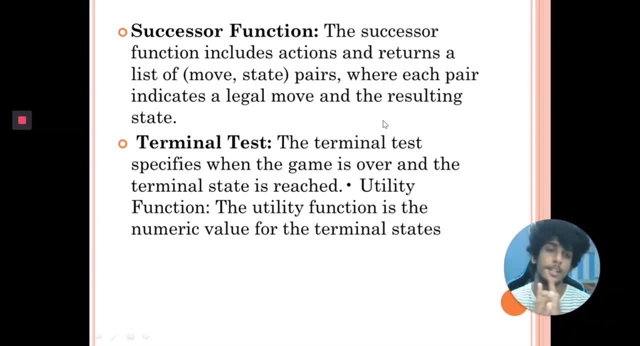 and one. so zero is while the game is running and the one is while the game is terminated. so if the value is one, you'll get the value in the screen as game over. so game over states that the game is over and you have lost and you have gained anything else. so yeah, okay, then we'll move on. 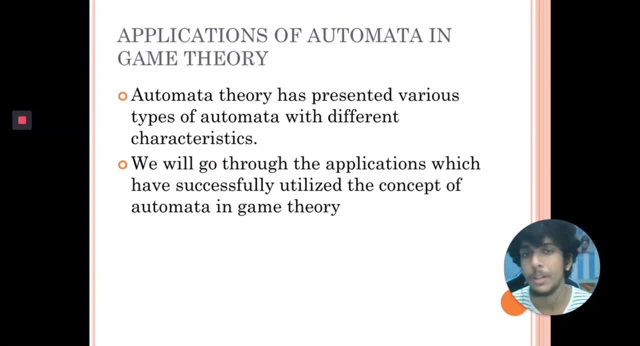 to the applications of automata in game theory. okay, automata theory has presented various types of automata with different characteristics, as you know about. so now we'll go through the applications which have successfully utilized the concepts of automata in game theory. there are various, numerous automata. i mean numerous concepts, which 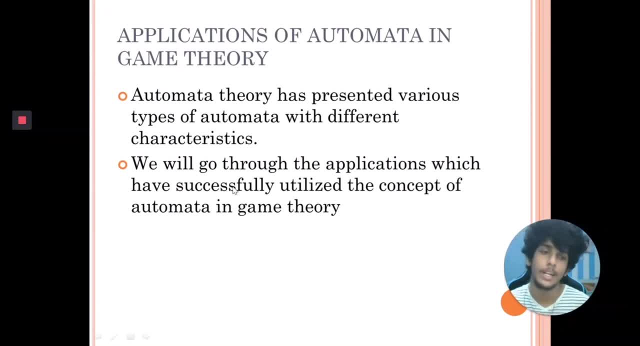 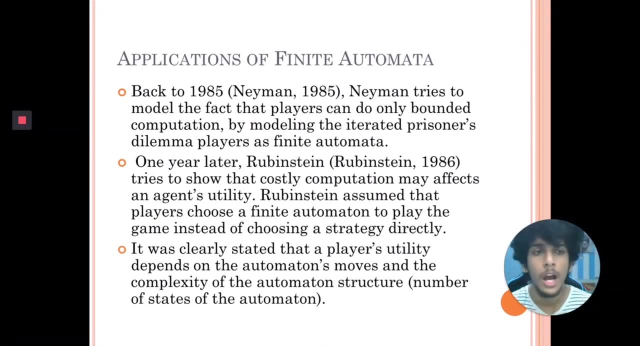 adaptively adapted the study of automata in game theory, so we'll look on to that in the following example. so i have chosen some. i mean i have split this into three types: applications of finite automata, applications of adaptive automata. applications of cellular automata. applications of cellular. 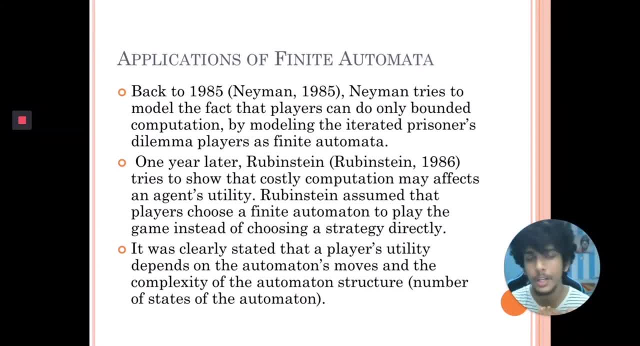 automata hasn't been defined in our presentation, as research is going on in cellular automata. it is the future of game theory, so now we are currently applying finite automata and adaptive automata, cellular automata and adaptive automata. automata is the thing where people integrate and they are currently working on cellular automata. 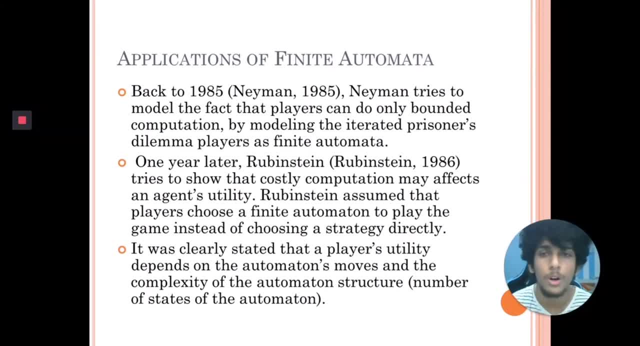 so, uh, we'll now look on the applications of finite automata. so okay, back in 1985, neiman neiman tries to model the fact that players can do only bounded computer computation by modeling the iterated prisoners dilemma players as finite automata. so this starts in the year 1985, back in 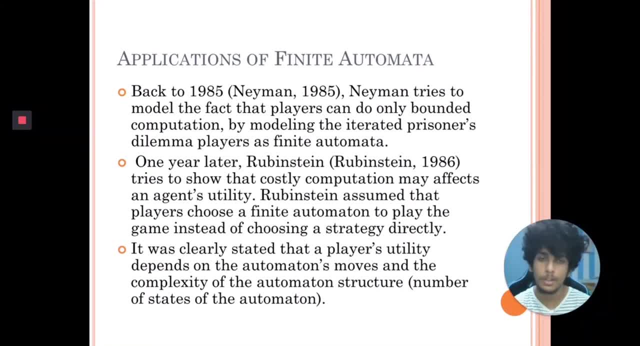 1985. so neiman neiman is the author. i mean, neiman neiman tries to model the fact that players can do only bounded computation by modeling the iterated prisoner dilemma as finite automata. so uh, back in 1985 neiman tries to model the fact. i mean he tried to state that only the bounded computation 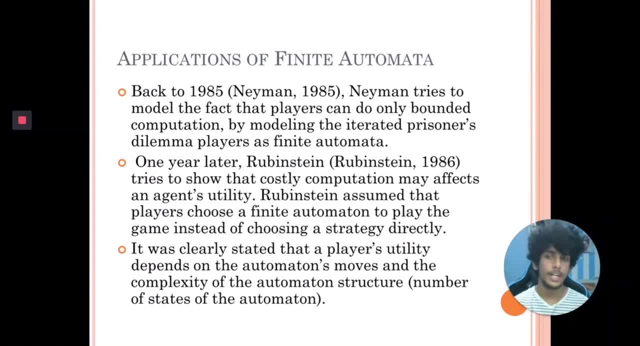 by modeling the iterated prisoners dilemma as finite automata. so finite automata was the thing that was approached and adapted by the players back in 1985, the 18th or 19th century. so that was the start of applying the automata and game theory. 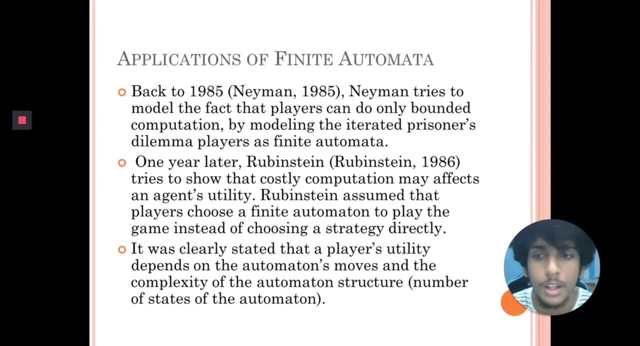 one year later, rubinstein. rubinstein tries to show the costly computation may affect an agent's utility. rubinstein assumed that players choose a finite automaton- automaton to play the game instead of choosing a strategy directly directly. so rubinstein assumed that, uh, players can use a. 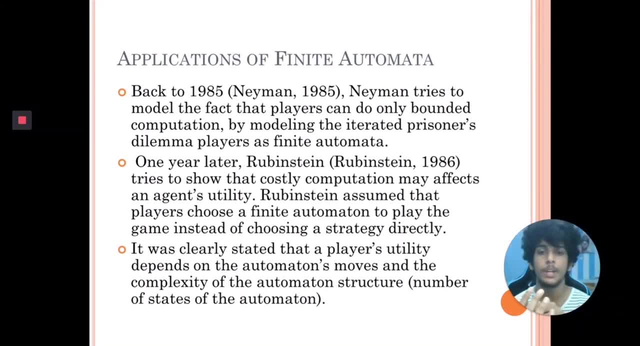 finite automaton to play the game, instead of choosing. i mean, he stated that, instead of using, an automata, can be used which eases the work of the players instead of choosing a strategy directly. and it was clearly stated that a player's utility depends on the automaton's move and the complexity. 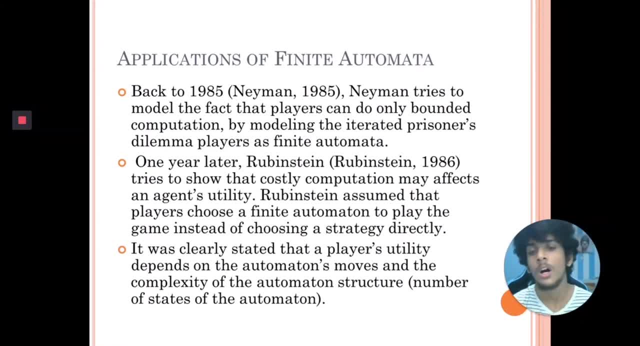 of the automaton structures. uh, complexity of an automated structure is nothing but number of states in automaton. so it was clearly stated that players utility depends on the automaton moves. uh, rubinstein stated that if a player moves it is up to his thing where he applies any automata and the thing moves. he didn't uh, actually say that you. 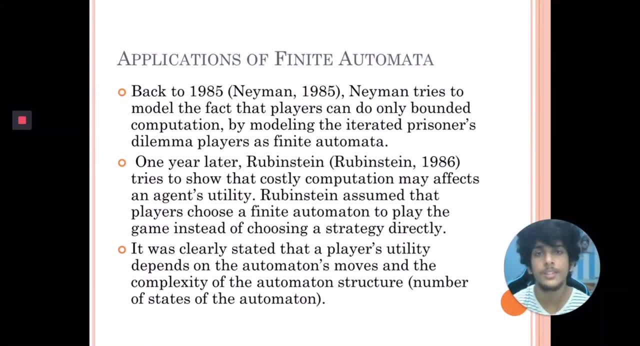 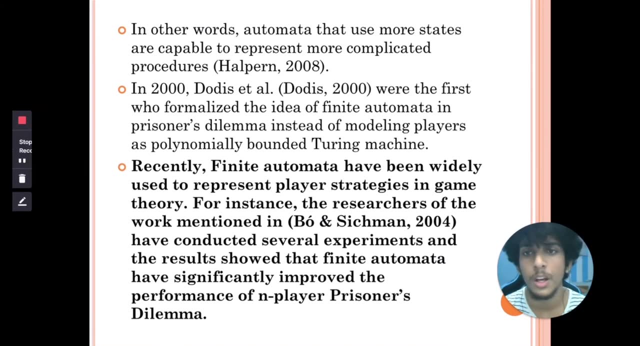 have to apply any strategy, whereas he said we can adopt automata in applying a game theory. so this was the first breakthrough of applying finite automata in a game theory, and in other words, that use more complicated states are capable to represent more complicated procedures. uh, in 2000, uh dodis were the first who formalized the idea of finite automata. 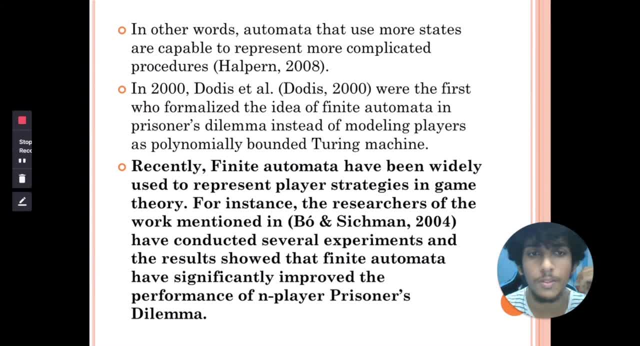 in persons, i mean in the prisoner's dilemma, instead of modeling players as polynomially bounded turing machines. so in 2000, dodis was the. i mean, they were the people who formalized the idea of finite automata in a prisoner's dilemma, instead of modeling players as polynomially. 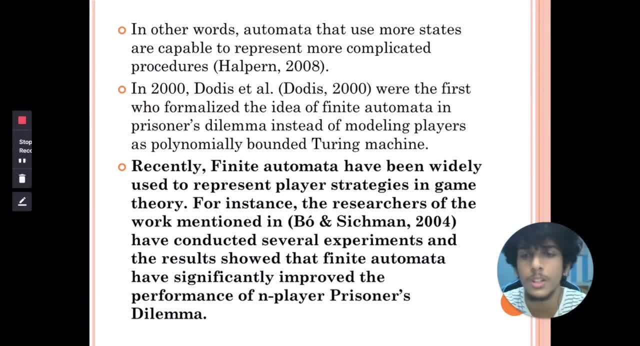 bounded turing machines. so turing machine was the thing which was found in the year 1998 and they integrated the fact and started to- uh, i mean started to integrate that thing in the year 2000. so recently, finite automata have been widely used to represent player strategies in game theory. 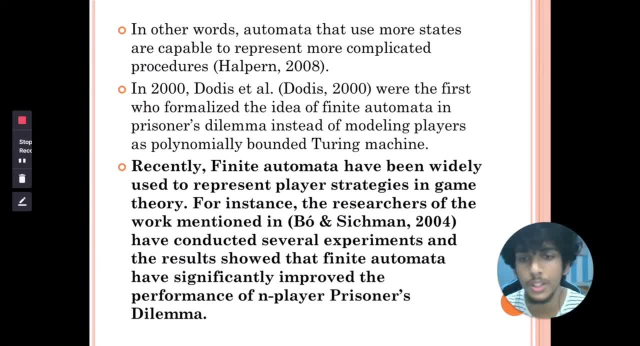 for instance, the researchers of the work mentioned in the bowen switchman 2004 have conducted several experiments and the results show that finite automata have significantly improved the performance of n player prisoners dilemma. so the prisoners dilemma was found in the year 2000. 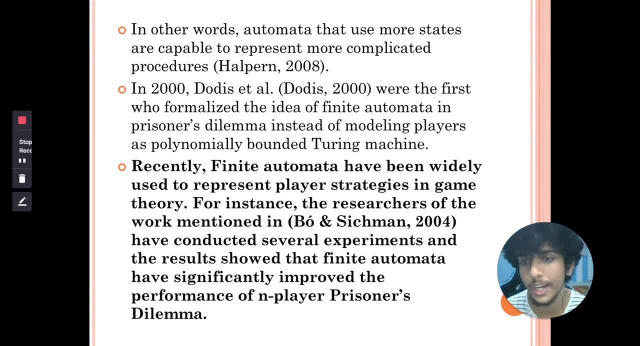 and recently, finite automata have been widely used to represent player strategies, for instance. the researcher have also mentioned that. i mean they have conducted several experiments and the results showed that finite automata have significantly improved the performance of n player. prisoners dilemma, yeah. however, finite automata are found to be efficient in representing simple strategies. 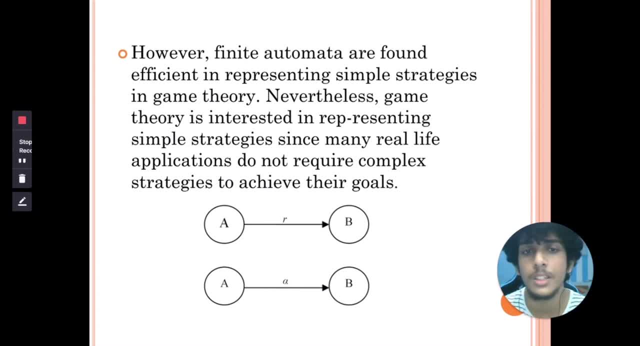 in game theory. nevertheless, game theory is interested in representing simple strategies, since many real life applications do not require complex strategies to achieve their goals. so back in the year they suggested that using finite automata would make the process more simpler. and uh, as people say, real life applications do not require complex strategies to achieve their 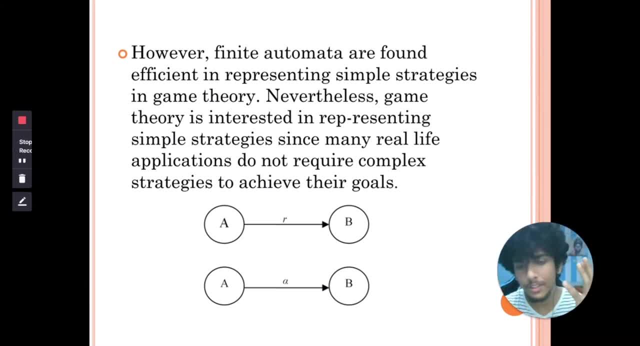 goals. so, uh, achieving the- they people achieve their goals using the finite automata. so finite automata is nothing, but there will be- i mean there'll be- finite number of states in each automata. so that is the basic definition of finite automata, and next we'll move on with 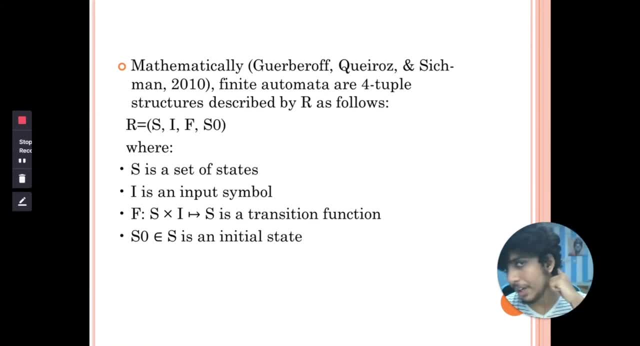 the. i mean we move on with the problem which was defined by guo, befroth and queros and switchman in 2010, which stated that how game theory was exactly applied using automata. so, mathematically finite automata are four tuple structures described by r as follows. as we know, a finite automata can be: 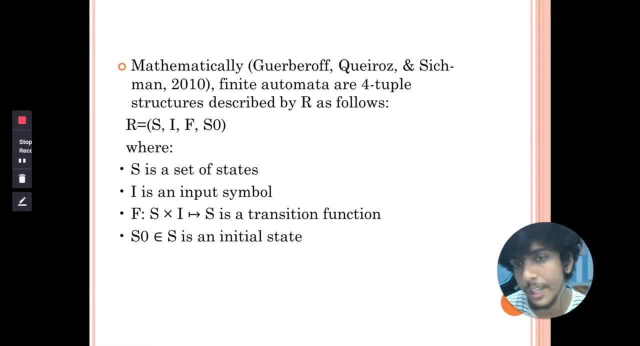 represented by s, i, f and s naught, so s is a set of states. i is a input symbol, f is equal to s cartesian product of i, which, where s is a transition state, s naught belongs to s, where s naught is the initial state. so we'll move on to the structure of automata. so, uh, i mean the 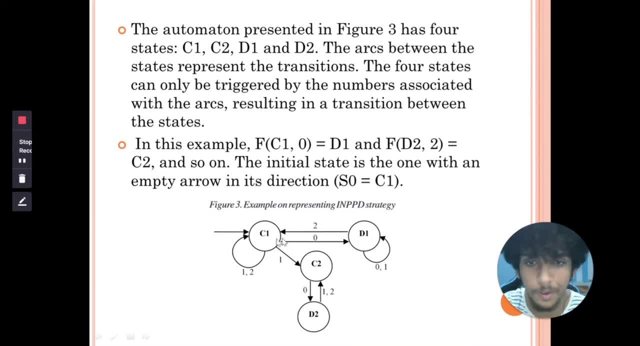 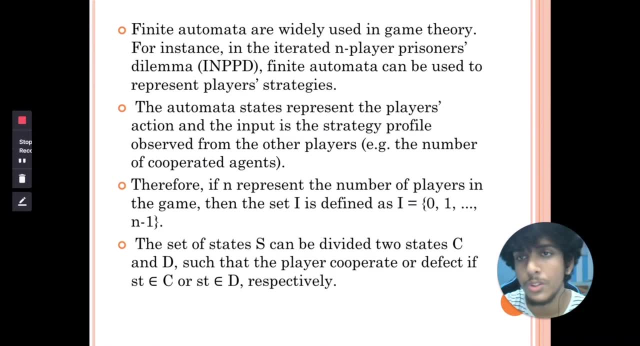 structure of automata is explained over here, but before coming to the figure, we'll understand what this prisoners automata defines. so finite automata are widely used in game theory, for instance the in the iterated n player prisoners dilemma, finite automata can be used to represent player strategies. 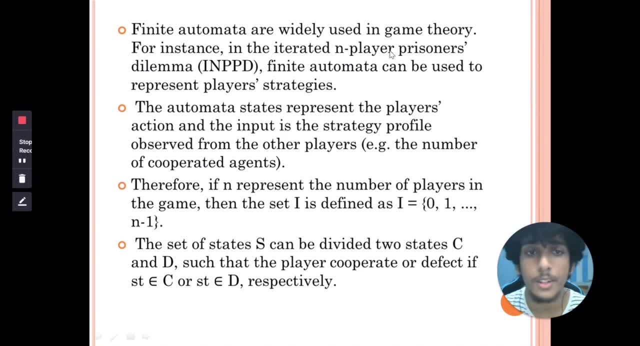 the automata represents the player's action and the input is the strategy profile observed from the players, example, the number of cooperated agents. so this automata state represents a player action and the input strategy profile. so therefore, if n represents the number of players in the game, then the set i is defined as i is equal to 0: 1 up to n number of players, which is 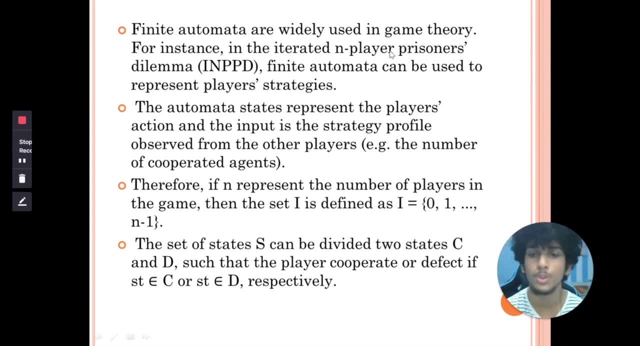 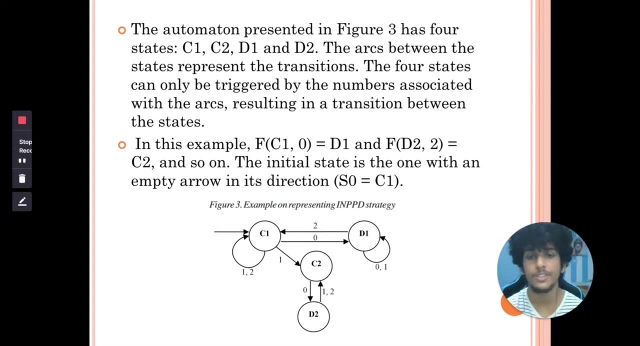 n minus 1. so the set of states s can be divided into two states, c and d, such as the player, cooperates or defects. if statement belongs to c or this, i mean the state belongs to c or the state belongs to d respectively. so the automata presented in the figure 3 has four states: c1, c2, d1, d2, the arcs. 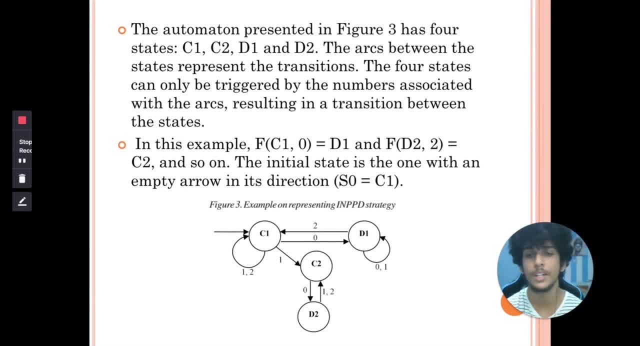 between the states represent transitions. so, as we know, that the state to state transition happens in finite automata. so the four states can only be triggered by number of associated with, i mean the numbers associated with arcs resulting in a transition between the states. so, as we see over here, if c1 is given a value of 0, it goes to d1 and d1 is given a value. 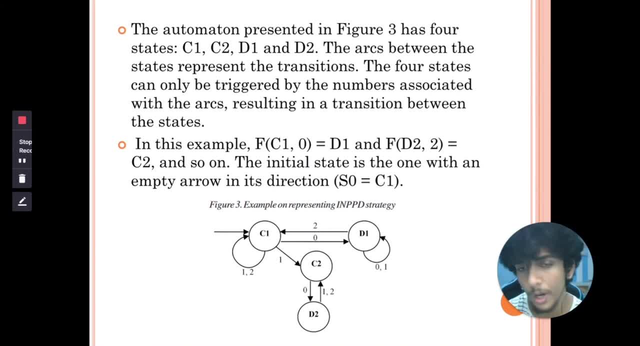 of 2, it comes to d2 and there are self loops with 1 and 2 in c1 and d1. but the d1 self loop occurs when it is given 0 and 1 and c1 is given 1, it goes to c2 and while c2 is given 0, it goes to d2. 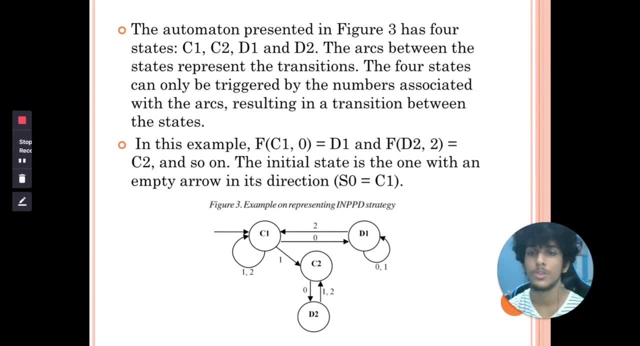 while d2 is given 1 and 2, it comes to c2. so in this example of c1 comma, 0 gives d1. as we stated that when f- i mean when c1- is given a value of 0, it goes to d1. 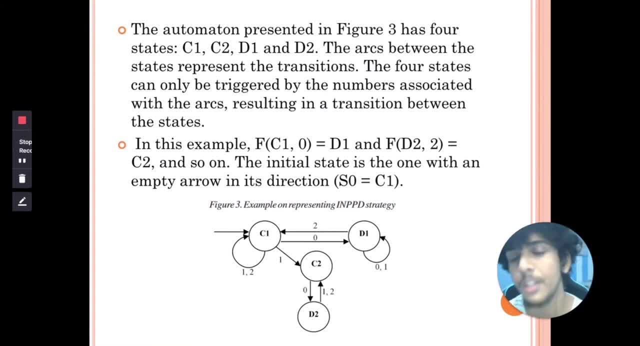 that is what explained, that is what which is explained in the mathematical form over here. and f of d2, f of d2. where d2 is given a value of 2, it comes to c2. so this is the major example of the transition arcs which are explained over there in the mathematical form. so the initial state is: 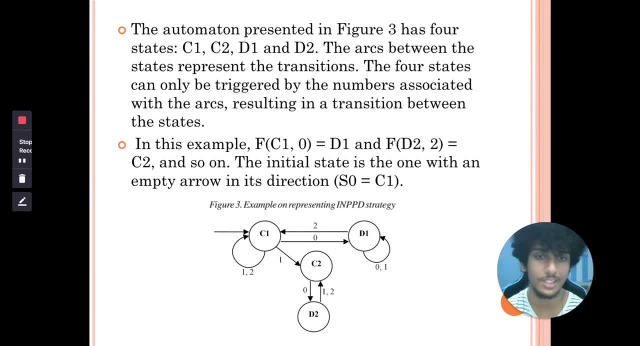 the one where an empty arrow in its direction- so that is s naught- is equal to c1. so, uh, while you see over here, uh, there is a value of, i mean this is the initial value. where, uh, it's not, i mean this is an input state with initial value. so that is, this is called as initial state, where the automata 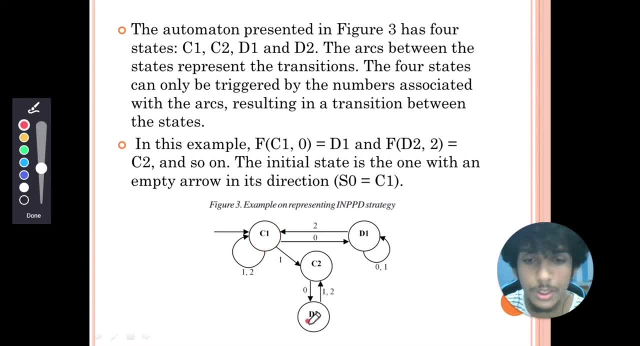 is getting completed in two states. they are d2 and d1, so we call this as final states, as i have not mentioned over here the final state. but if you, uh, i mean if you give double circle to the states, that is considered as the final state. so yeah, we'll. 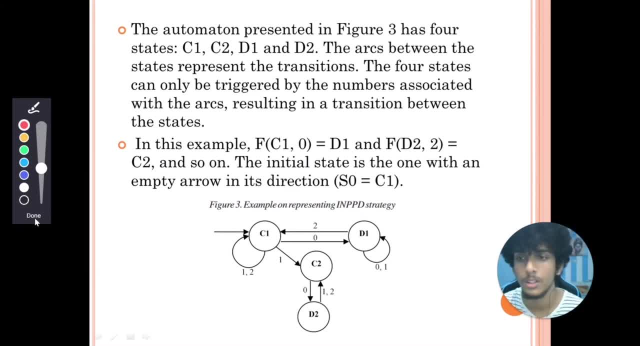 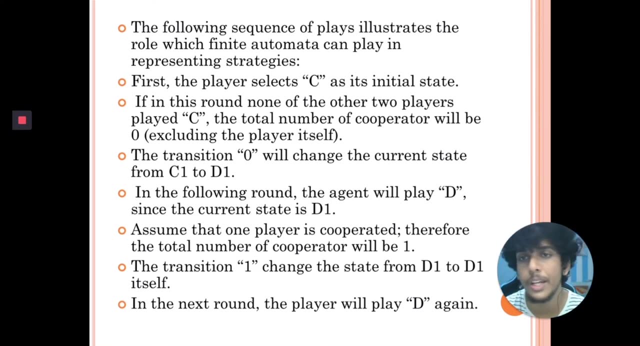 move on forward. so okay, so i'll explain what is given over here, i mean, i'll explain the process of what is happening over here in this automata diagram. so the following sequence of play illustrates the role which automata can be represented in different strategies. first, 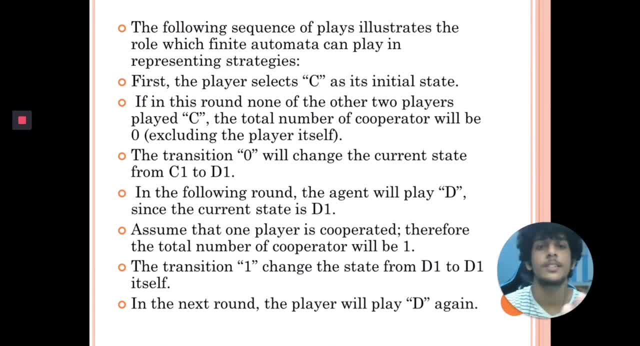 the player c select c as initial state. so the player selects the c as the initial state. if in this round none of the other players cooperates, the value is taken as zero and the total number of cooperators will be zero. the transition zero will change the current state from c1 to d1, as we saw in the above diagram and in the 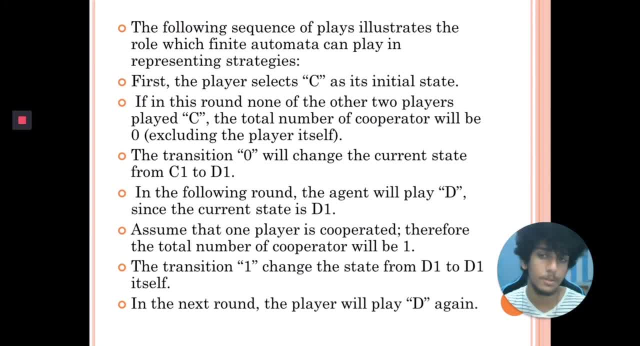 following round. the agent will play d as he moves from c to c1 to d1 and the current state of the player is d1. so assume that one player is cooperated. therefore the total number of cooperator will be one. as the people move will move from d1. so as the cooperator state is one, the value will remain. 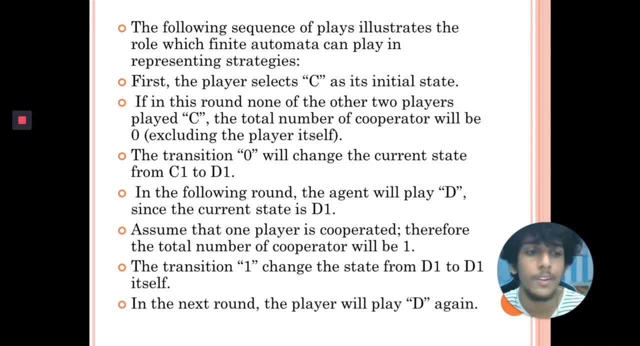 on d1. so in the next round, if the player will play d again, uh, the cooperator value will get updated to a value of two. so if it gets updated to a value of two, it will move to the d2 state. so that is what explained in this example. so, however, using finite automata as model language, 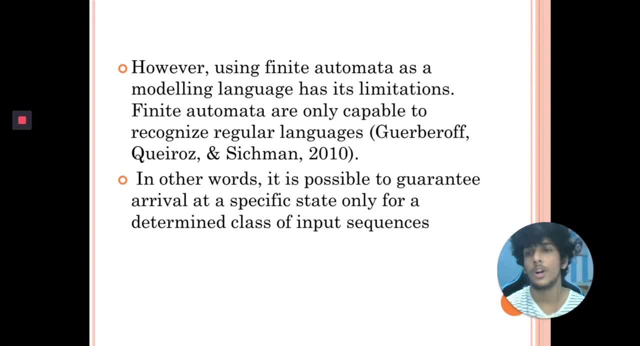 has its limitations. so not only i mean: why did the people move on from finite automata to adaptive automata? the basic uh idea behind that was: using finite automata as a modeling language has its own limitations. finite automata are only capable of recognizing regular languages, whereas there are 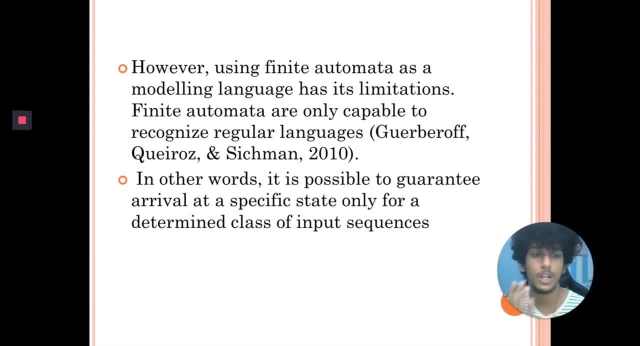 many languages like contact-free language content, uh, free grammar and chomsky normal form and there are many things like that. so we have to develop the another automata, such as pushdown automata, non-deterministic pushdown automata and things like that, to develop a language. so, in other words, 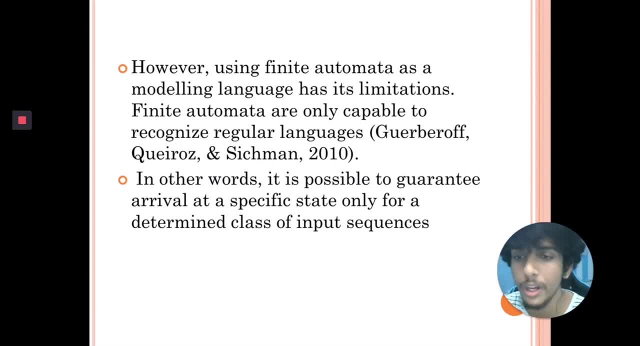 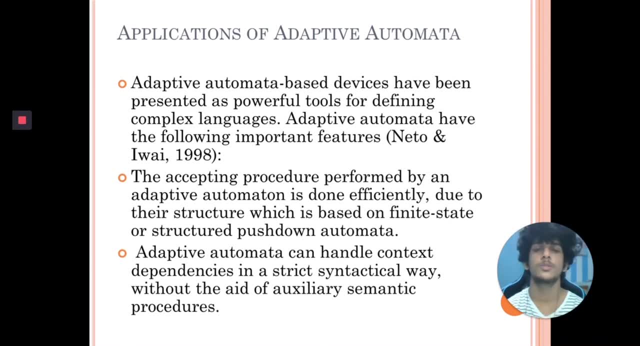 ninety: arrival at a specific state only for a determined class of input sequences. yeah, so next we'll move on with the applications of adaptive automata. so now we have completed the applications of finite automata, then people moved on with the applications of adaptive automata. i mean they. 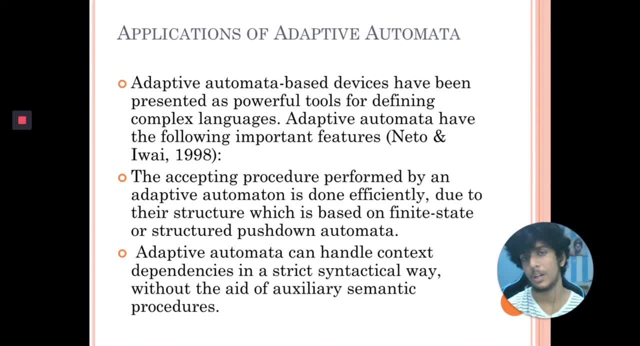 moved on with adaptive automata. so adaptive automata is nothing but adaptive automata based devices have presented as powerful tools for defining complex languages. adaptive automata have NITO. I mean adaptive automata have the following important features which are given by NITO and: 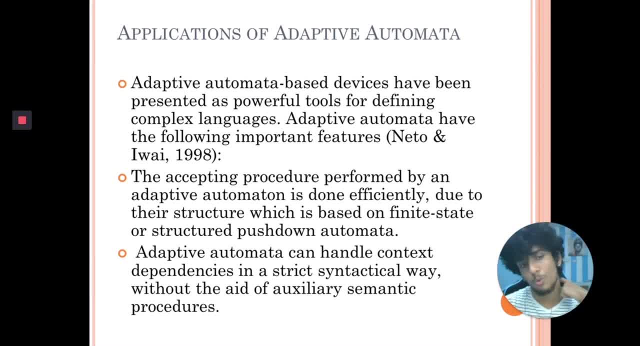 EVA in the year 1998.. So what did they say? That is the question. So they said that the accepting procedure performed by an adaptive automaton is done efficiently due to the structure, which is based on finite state or structured pushdown automata. Adaptive automata can handle context. 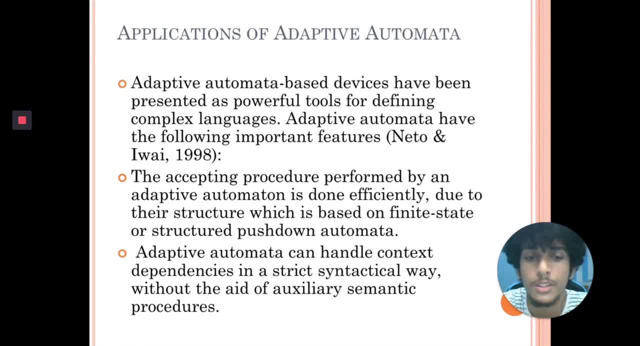 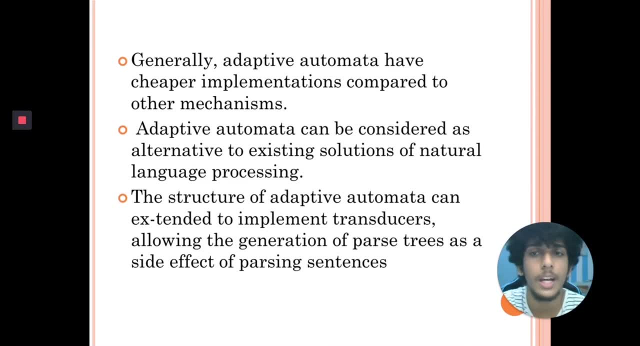 dependencies in a strict syntactical way, without the aid of auxiliary semantic procedures. Generally, adaptive automata have cheaper implementations compared to other machines. Adaptive automata can be considered as alternative to existing solution of natural language processing. The structure of adaptive automata can be extended to implement transducers. 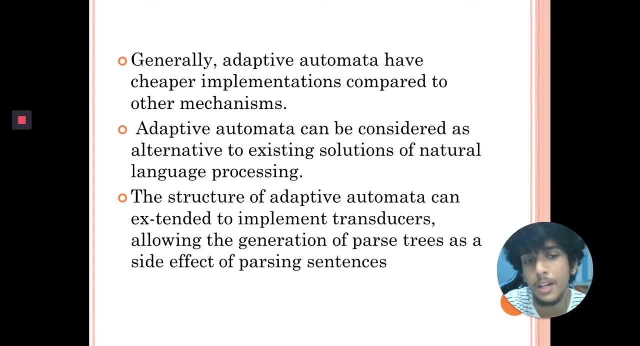 allowing the generation of parse tree as a side effects of passing sentences. So, basically, generally adaptive automata have cheaper implementations compared to other mechanisms. That is the question. So what did they say? That is the question. So what did they say? 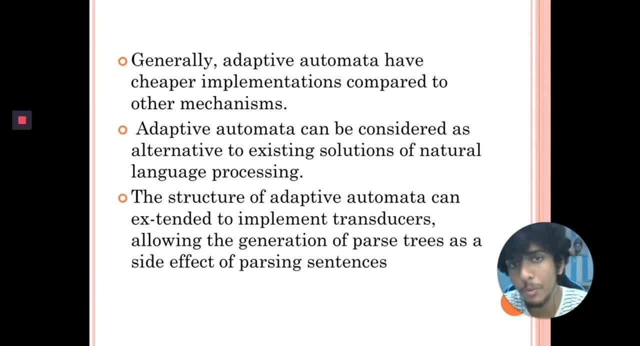 That is why people moved on from adaptive automata. I mean, that is why people moved on from finite automata to adaptive automata, as the applications and the implementation is cheaper than other mechanisms such as finite automata. So adaptive automata can be considered as alternative to. 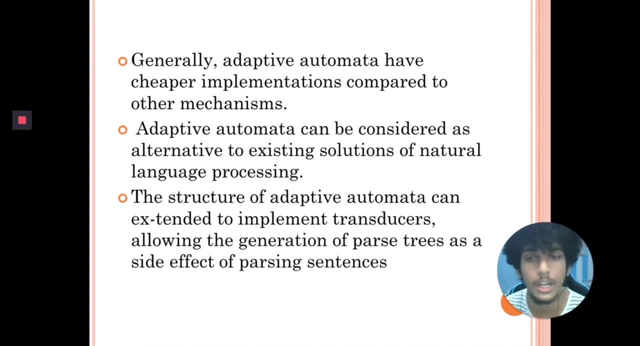 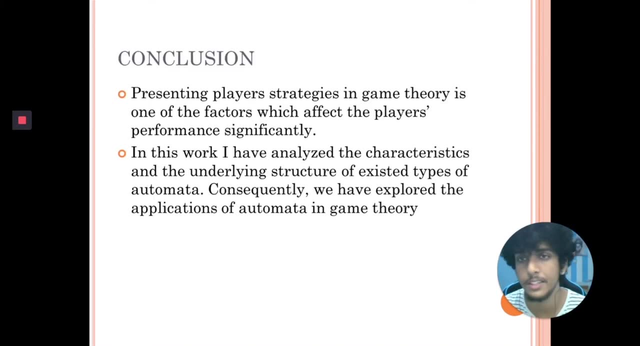 existing solutions of natural language processing So the structure can be used to implement transducers allowing the generation- I mean adaptive. automata uses the- I mean uses the help of parse trees as a side effect for passing sentences in lexical analysis. So the basic conclusion of automata in game theory is presenting player strategy in game theory is one. 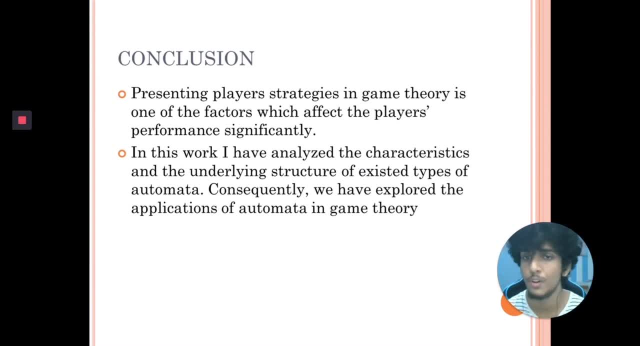 of the factors which affects the player's performance significantly. So strategies in game theory are the only major factors which affects the player's performance significantly. So we are trying to change the strategy with the help of- I mean trying to overthink the strategy with the. 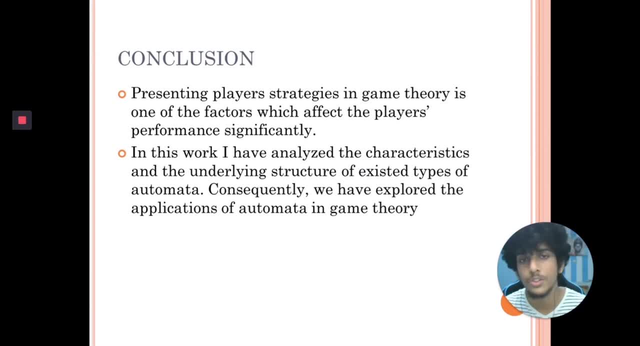 help of another factor which is called as automata. So in this work I have analyzed the characteristics of the underlying structure of existing types of automata, such as finite automata, adaptive automata, and I am currently working on- the people are working on how cellular automata is used to. I mean how cellular automata is used to is used in game theory to implement the strategies over there. 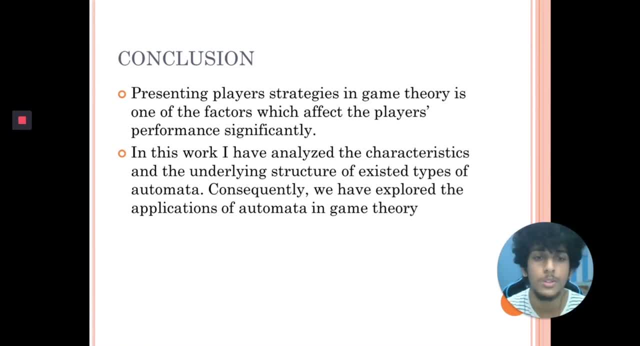 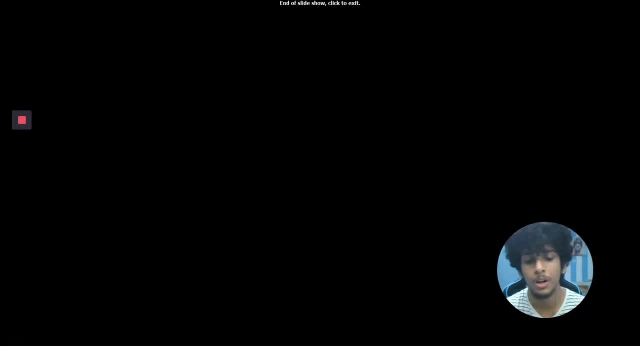 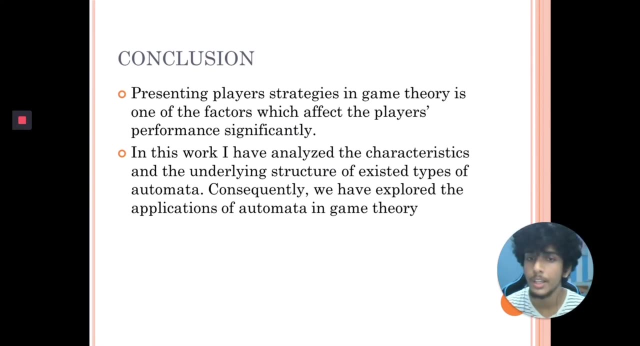 Consequently, we have also explored the applications of automata in game theory. So that's it for my presentation. Thank you, Hope, hope this application of automata in game theory is useful, Well presented by me. and yeah, that's it from my side. Bye, bye from Abhishek.